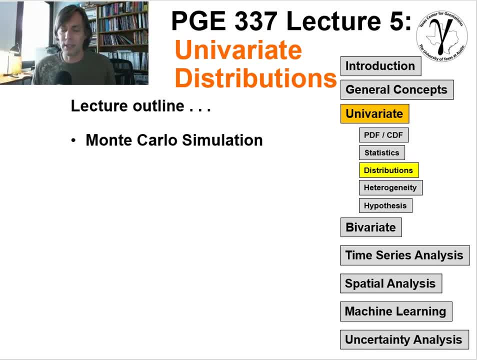 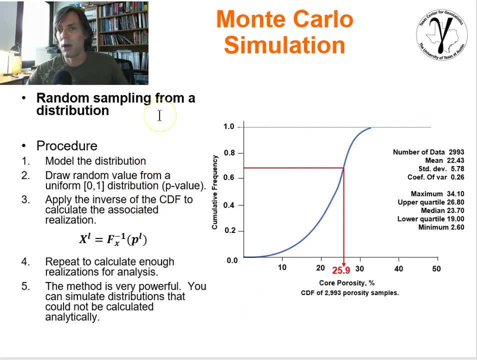 directly with the data. Let's get into Monte Carlo simulation. So Monte Carlo simulation is an extremely powerful numerical method. It's been used to solve very difficult and challenging problems. From the first slide it will not be apparent why that's the case. but don't be. 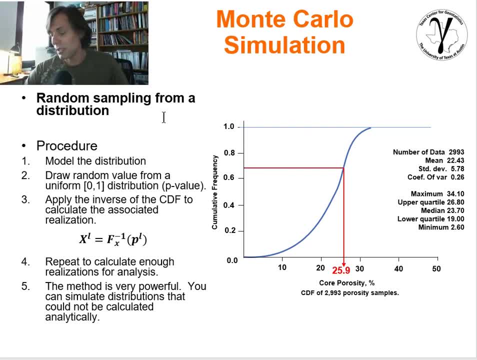 disturbed by the simplicity of it. In fact, we'll show you an example of what we can do with it, but of course there's much more complicated things that we can do. So what is Monte Carlo simulation? Monte Carlo simulation is simply random sampling from a distribution. That's it. 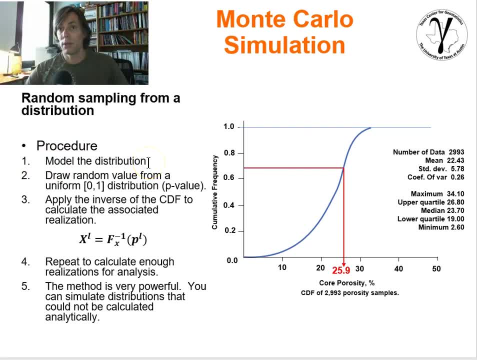 So the procedure would be: first you model the distribution so that distribution could be represented by this CDF, right here with the blue line. This is our distribution, a continuous representation of that full CDF. Then what you do is you draw a random value from a uniform zero for the min. 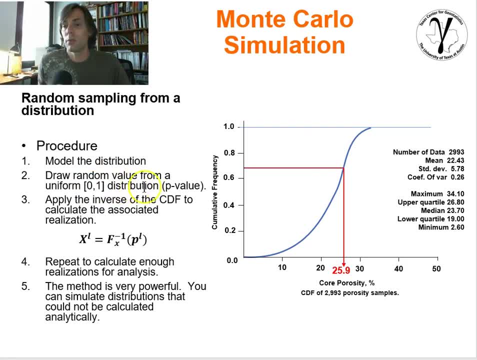 one for the maximum value distribution. This is your p-value. This is the p-value that you're going to use to now draw from that distribution. Then you apply the inverse of the CDF operator to calculate the associated realization of the value of interest from that distribution. So p to l is our p-value realization. We drew it. 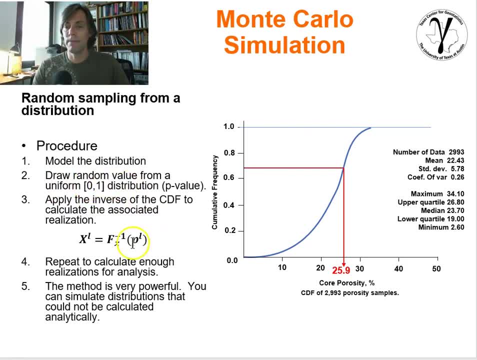 randomly from a uniform zero to one distribution. Now we apply it to the inverse of our CDF and the result will be a realization from the property distribution. So graphically we can denote it like this: Here's our axis for the cumulative. 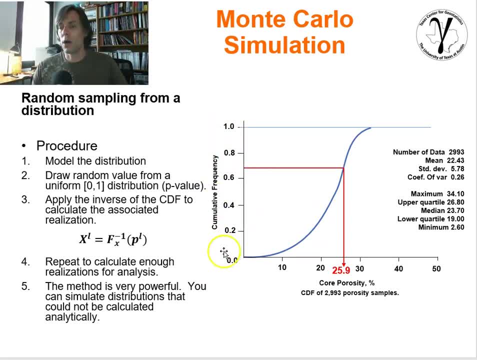 probability from our CDF. We draw a random value uniformly distributed between zero and one. We've got a value of about probably something on the order of about 0.67 or so We come across. this is the inverse CDF operator. We get to the function, we go down, and so we have drawn a. 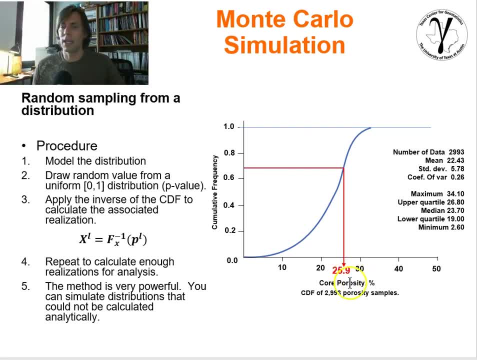 value of 25.9% porosity from our distribution of core porosities that were provided to us by almost 3,000 data. That right there is a Monte Carlo simulation. Now, typically one realization is not enough. You will repeat this and calculate multiple realizations using. 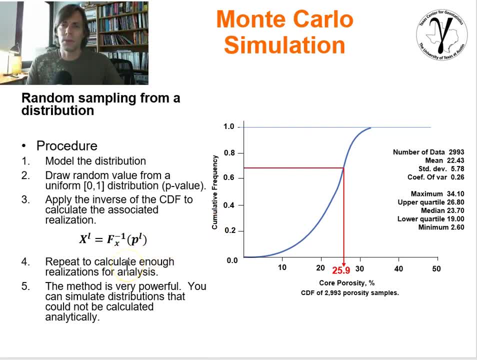 Monte Carlo simulation. Until you have enough realizations, you've sufficiently sampled the problem that you can complete your analysis. So you're going to have a value of 25.9% porosity from your analysis. for whatever workflow you're working with, The method is very powerful. 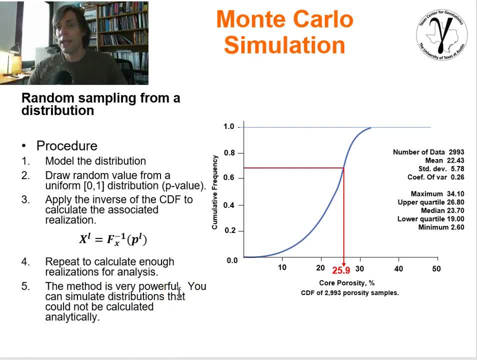 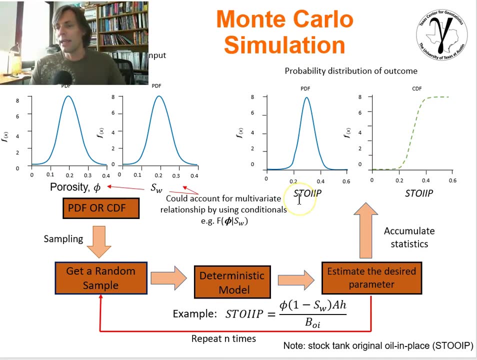 You can simulate distributions that you would not be able to calculate analytically, And I'll show you an example right away of a case of that. So here's an example of a Monte Carlo simulation to assess the amount of oil in place. Oh, excuse this. So basically, these right here. 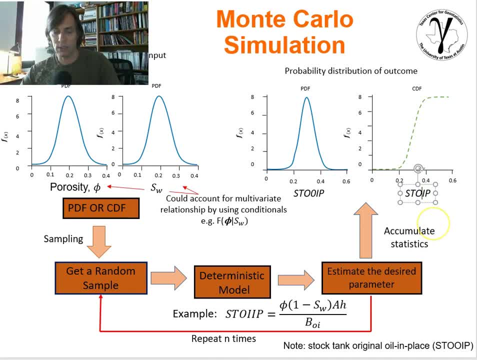 our stock tank. original oil in place is what we want, And so we're going to go ahead and calculate that using the oil in place equation shown right here. We're going to use the average porosity, which tells us about how much of the rock is pore volume available to put fluids in it. 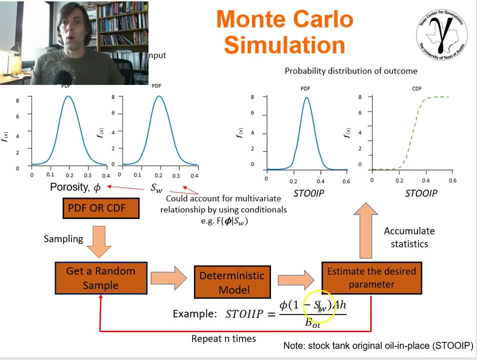 We have the saturation of oil or hydrocarbon, which would be one minus the saturation of water, And we have the area and the height of the reservoir, which gives us the volume of the reservoir. This B factor here is going to account for the fact that the conditions 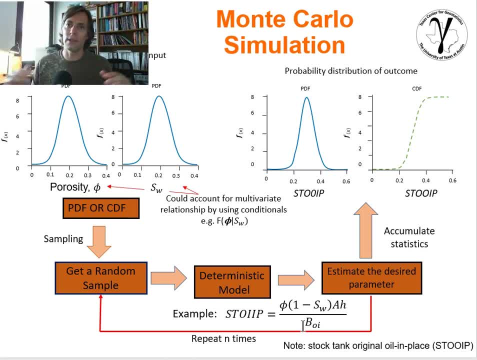 are different. in situ versus at the surface. You may have the expansion of a gas or whatever it might be. Well, this is oil, So you might have a change in the volume as you're coming up from high pressure at the subsurface to the surface, which has low pressure. So we're accounting for. 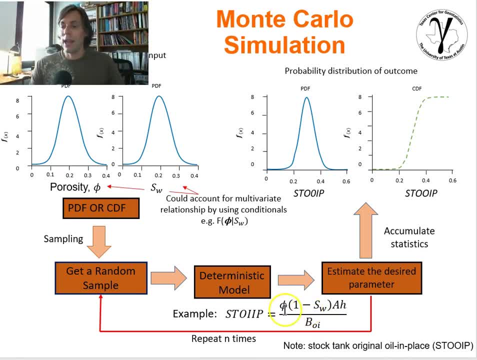 that with the B factor. Now you could imagine that the average porosity is uncertain. You only have sampled like one trillionth of the reservoir. You often don't have enough information available to you, And so there's an uncertainty distribution, And that's represented here by this Gaussian. 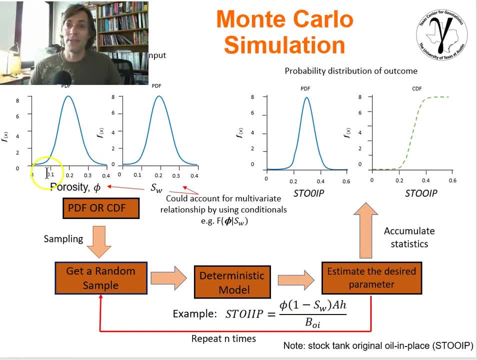 distribution. We put it as being very wide uncertainty, in fact, because it's going from effectively almost 0% porosity up to about 35% porosity. That would be unrealistically high, But this would be a very high porosity, And so we're going to go ahead and calculate that. 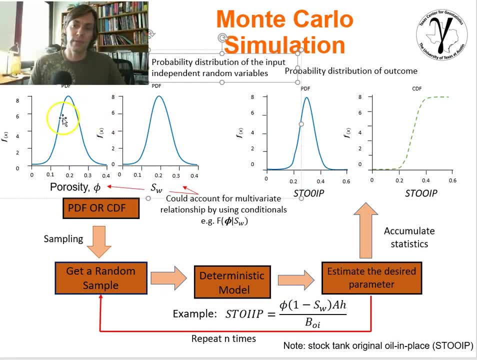 This would be the distribution of uncertainty for porosity. Saturation of water also has uncertainty. It may be heterogeneous, It may change locally, And we've also sampled that with very few data, And so we have uncertainty distribution with a mode, something around. 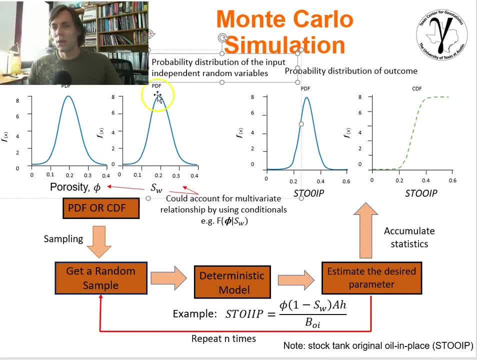 20% water saturation, And so these are both uncertain and we want to account for them. Now it would be very difficult to take this, this equation, and to put these distributions in and solve for exactly what this distribution should look like. In this case, it's a product. Yeah, it would probably be very difficult to do. 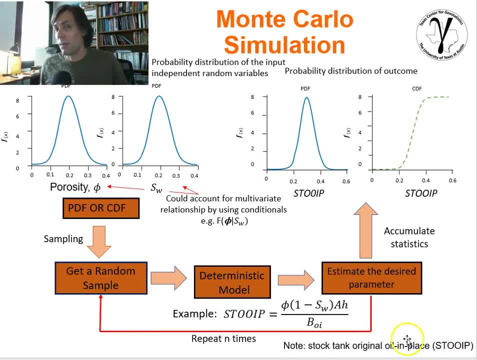 But using Monte Carlo simulation we can solve this problem. In fact, just to kind of give you a little bit more of a scope on what we could do with it, imagine if there was a square term or there was a square root term. 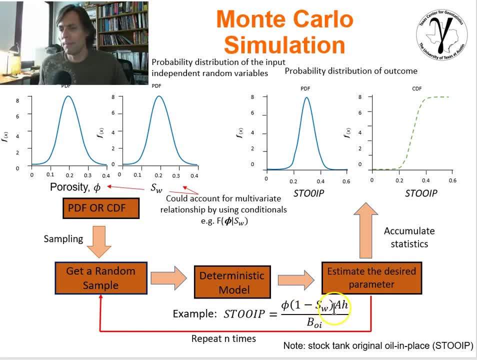 You know more complicated type of nonlinear operator within this equation. You could imagine you could not take the distribution of one variable, distribution of another variable, put them into this equation and solve for exactly what would be the distribution coming out. But Monte Carlo simulation is an avenue by which we can do that. So what do we do? We're going to 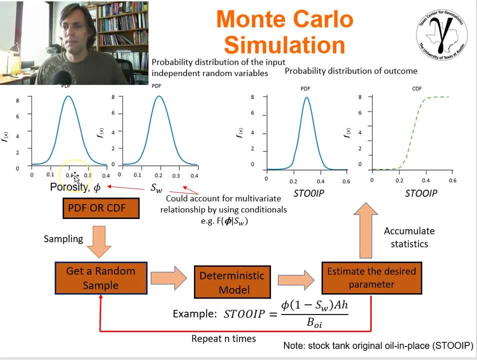 do Monte Carlo simulation from the porosity distribution, Then we'll do Monte Carlo simulation from the saturation Distribution. We take those two numbers, we substitute them into the equation, We get an estimate or realization of this output, And we then plot that or stored in the table. Then we 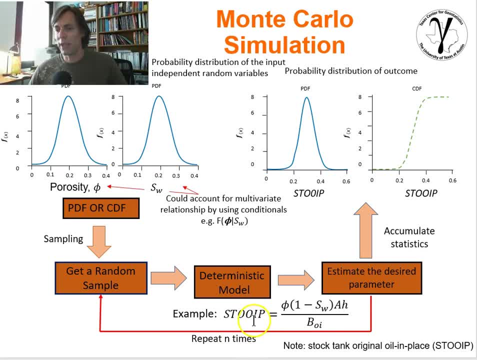 go ahead and we do another realization. from each one of these. We get another stoic. We go ahead and put that in the table And you do this until you have enough realizations of stoic that you're able to then get the entire distribution. 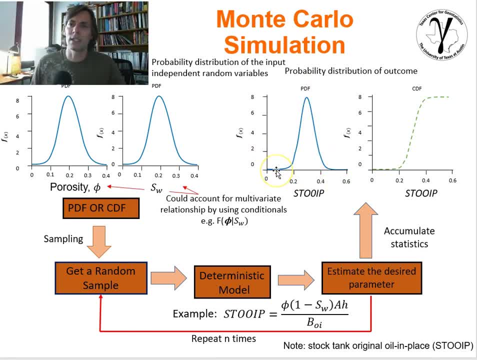 And then you can use that for an uncertainty assessment, making decisions about what you're going to do with development of the subsurface and so forth. Now this could be a lot more complicated. There could be a relationship between porosity and permeability, sorry. 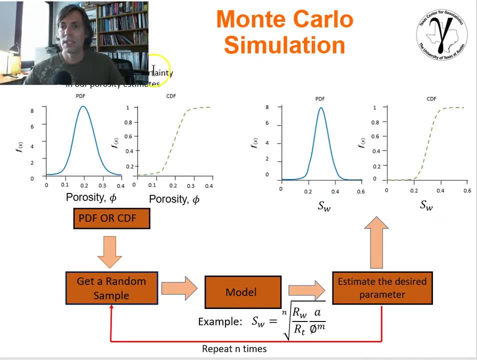 porosity and saturation, And so here's an example right here where in fact we have a relationship where saturation is related to the porosity by a pretty complicated form, And so we could do Monte Carlo simulation from porosity, Substitute that into the equation given. 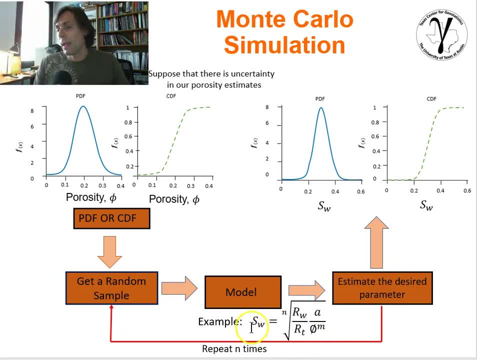 the other parameters are constants And we could calculate the associated realization of saturation of water. Repeat that many times. You would get a distribution of saturation of water. Or you could do it one time: Get a realization of porosity. Use this equation to get a realization of saturation. 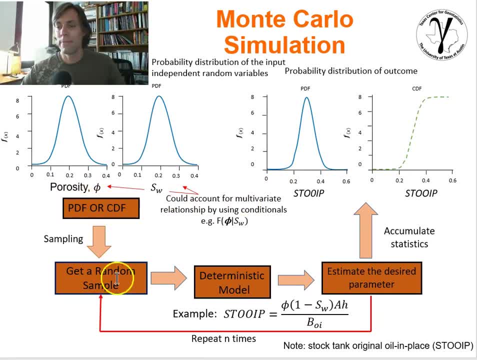 And then you would plug those two into this equation for a realization of stoic. So we have a hierarchical Monte Carlo simulation workflow where we first are simulating porosity using a relationship, a physics-driven relationship, to get a realization of saturation, And then taking both of them and getting a physics-driven. 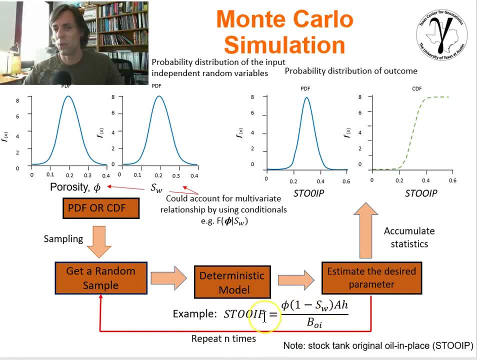 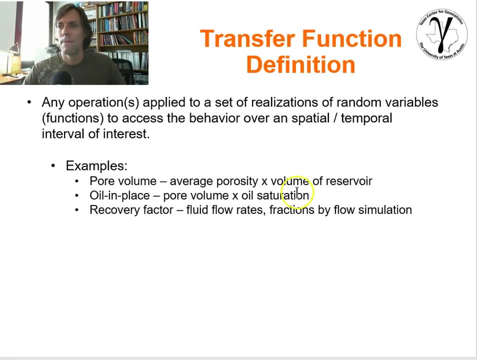 or really more geometric-driven realization of stoic, And you could repeat that many times until you get a full distribution of uncertainty for stoic, The. every time we're doing this, we're getting realizations of values And then we're putting them into a function. That's typically what we do in our workflows And we call that a. 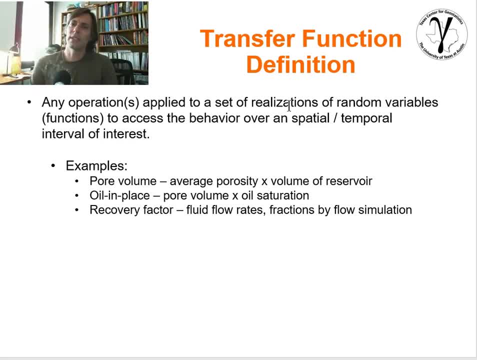 transfer function. In subsurface modeling, geostatistics, transfer function is defined as any operation or operations applied to a set of realizations of random variables and or random functions to access the behavior over and over again. And then we use the function and spatial or temporal interval of interest. 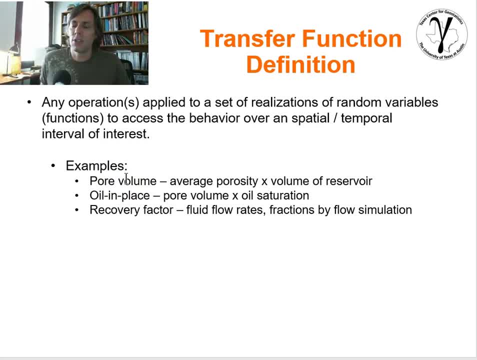 So what would be examples of that? Well, the Stoibe calculation just now was a calculation of the oil in place, And so we're concerned about calculating the overall pore volume and then using a saturation and some type of formation factor that's accounting for the in situ conditions, to get an oil in place. 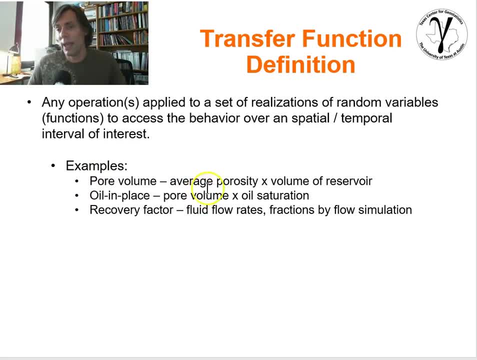 We could also just be interested in the pore volume, in which we'd be looking at the average porosity times, the reservoir volume, Or we could be working with recovery factor, in which case it would be a much more complicated transfer function. We would have a simulated heterogeneity field for porosity permeability. 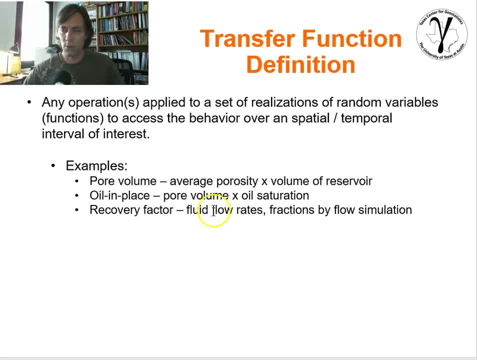 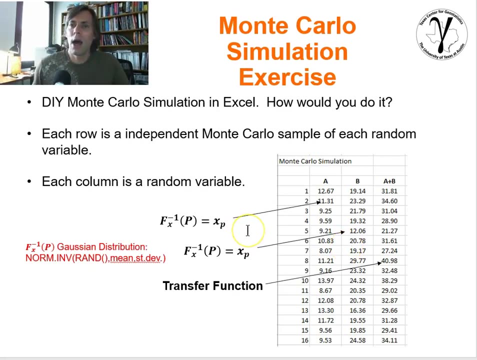 We would run physics-based flow simulation and we would get fluid flow rates and fractions of flow using the flow simulation. You know, do we have how much oil, how much water and so forth? Now how would you do it If you wanted to do DIY Monte Carlo simulation in Excel? 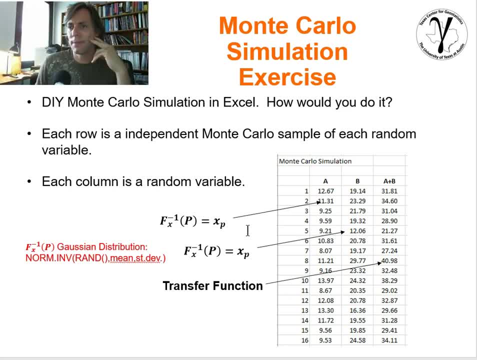 just try this out. Just try a very simple Monte Carlo exercise. The way I would set it up is I would have my variables in each column. I'd probably put a realization index here so I can just kind of track and see how many I have. 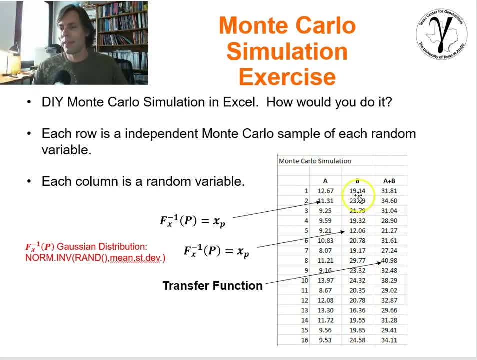 Variable A, variable B, and then I would have my transfer function. And so, for a very simple example, I could draw from a distribution a value of A. If it was Gaussian distributed in Excel, I could simply use the norm inverse brackets. 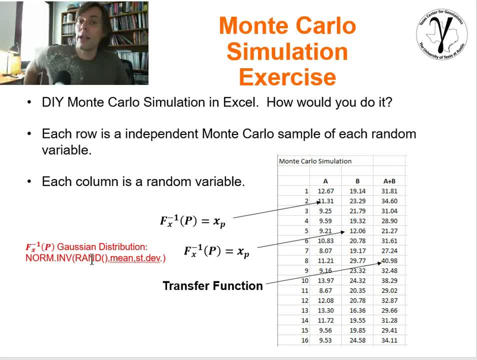 The first parameter should be the p-value. Now I want to draw a random value between 0 and 1, uniformly distributed, and so I use the rand operator. rand will give you a random number uniformly distributed between 0 and 1.. 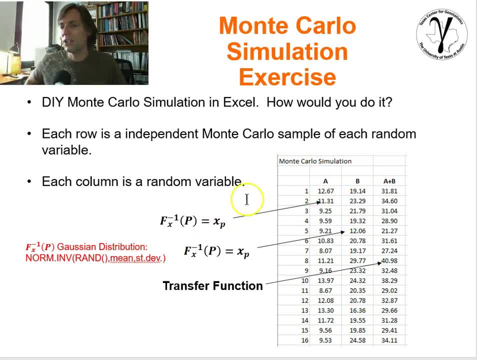 Then I specify a random value between 0 and 1, uniformly distributed between 0 and 1.. Then I specify the mean for A, the standard deviation for A, and then, if you just hit enter, you will get a Monte Carlo simulation from that Gaussian distribution. 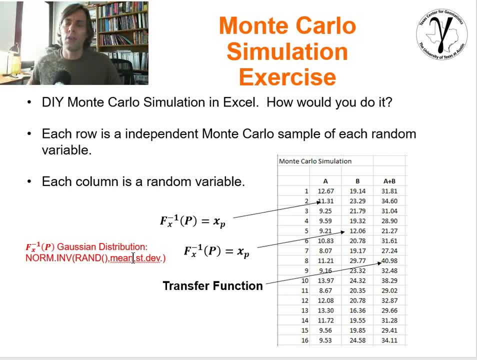 The rand operator will update every single time you hit enter or type in something new into your spreadsheet, so these numbers will effectively keep changing, dancing around. but it doesn't matter for our results, That's fine. Okay, so that's how we would set it up. 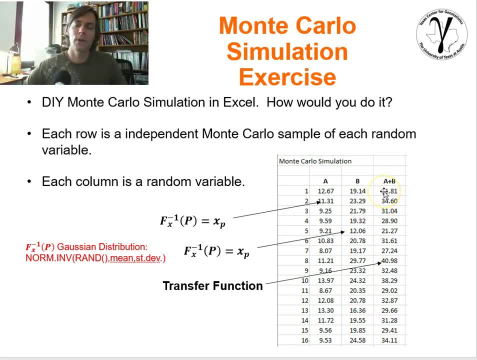 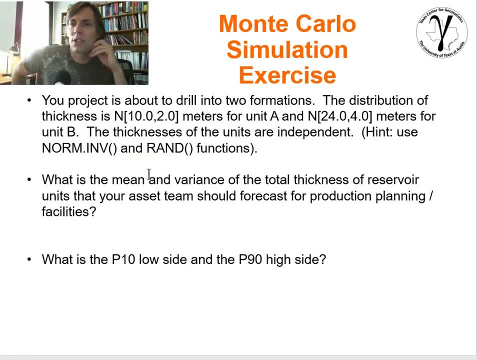 We'd do the other distribution for B, and if our transfer function was the same, if our transfer function was as simple as summing the two, we would put it like that. And so let's go ahead and try an example that looks just like that. 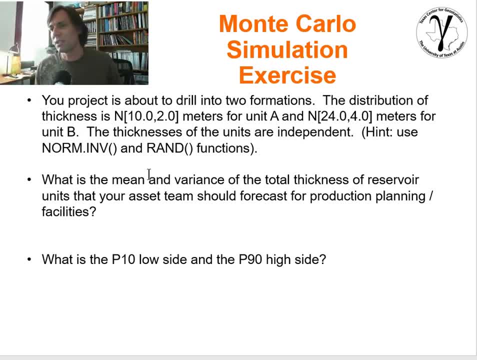 Just as simple as that. So your project is about to drill into two formations. The distribution of thickness of the first formation is mean of 10 meters, standard deviation of 2, it's normal or Gaussian distributed. The thickness of unit B has a mean of 24 meters. 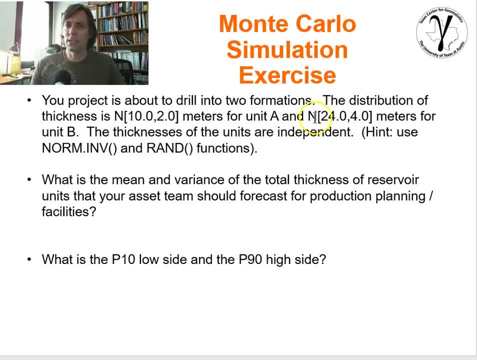 standard deviation of 4 meters, and I specify this Notice. I put an N here to indicate normal distribution, and then brackets mean standard deviation. That's it. The thicknesses of the units are independent, so you don't have to worry about modeling the correlation between the two. 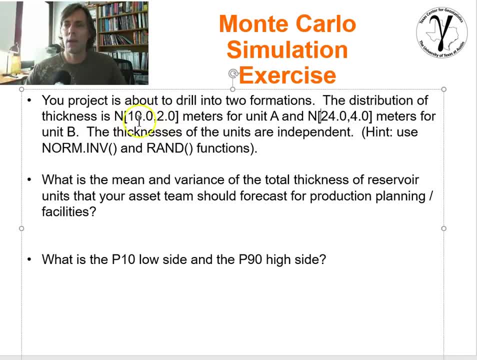 You just go ahead and get a Monte Carlo realization or simulation of A plus a Monte Carlo simulated realization of B. Add them together. Your transfer function is simply going to be addition. So what is the mean and variance of the total thickness of reservoir units? 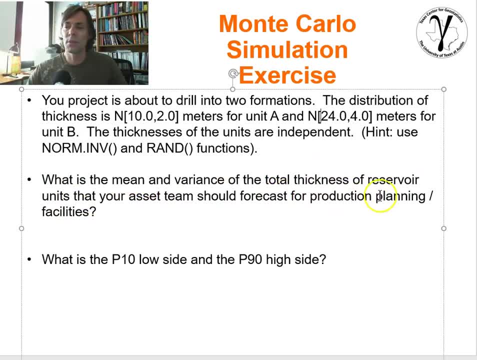 that your asset team should forecast for for the purpose of production planning and facilities. What's the P10?, What's the P90?? And so this would be a bit hard to do without Monte Carlo simulation. I'll show you: You can basically get it without doing it. 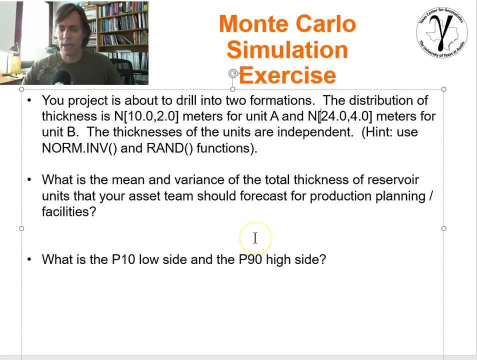 The problem is pretty simple. We can use a couple of mathematical concepts, but for the purpose of this exercise, we'll go ahead and use Monte Carlo simulation. So go ahead, put that into Excel and I will show you the answer in 3,, 2,, 1, and now. 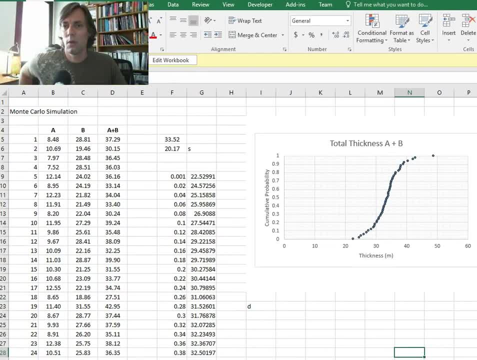 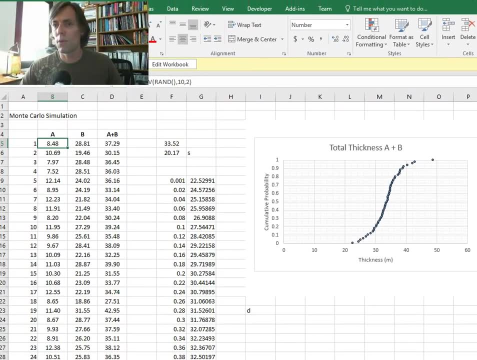 Let me just open up Excel, And so I've got Excel right here and I did just what I explained on the previous slide. In fact, let me move this down a bit more so you can see the command For A. I just took the normal inverse. 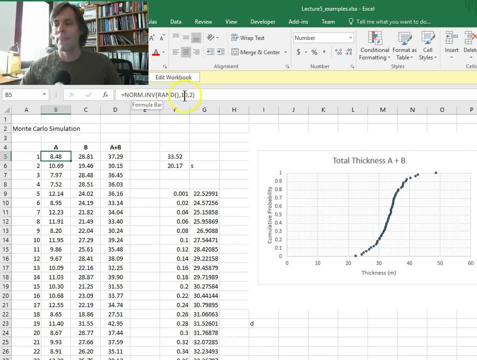 rand for a random value between 0 and 1,, 10 for the mean thickness of A, 2 for the standard deviation B, 24 and 4, random numbers. And all I did was take that command and just copy it down and paste. 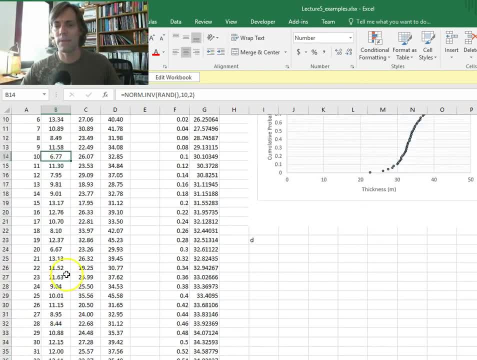 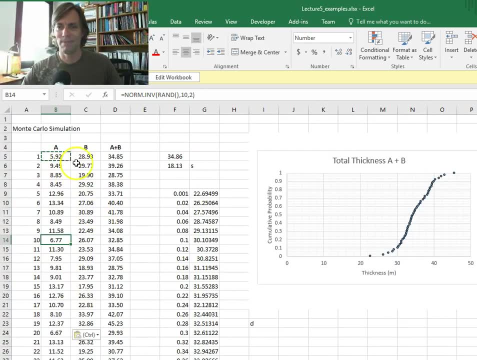 And when I did that, I have it in all the cells and I've done it for many cells. I think I've done it for 100.. Well, actually I got 103 realizations, Okay, So now I have those realizations. 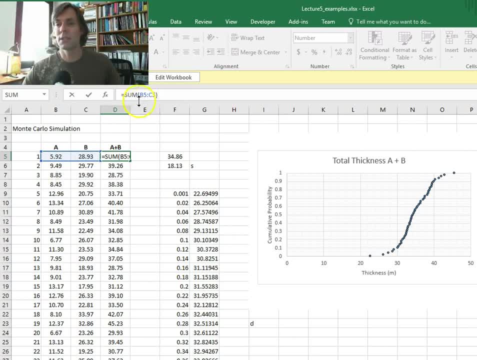 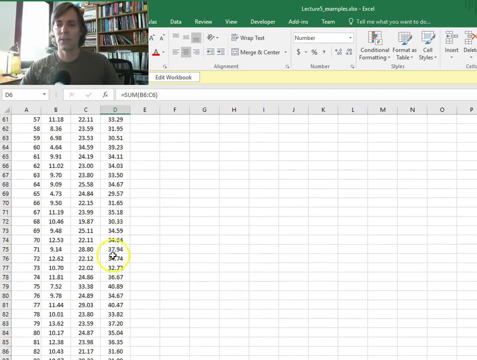 So in this page my transfer function is simply going to be the summation of the two, So I use the sum command. I could also just add them together, And now I have realizations of the output for my transfer function. 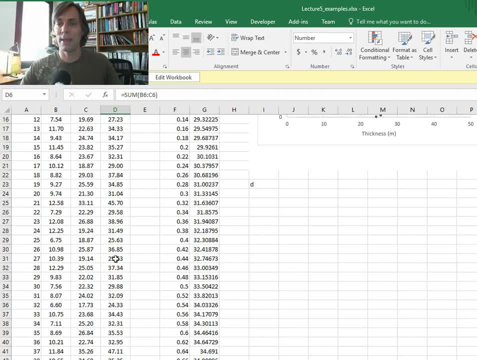 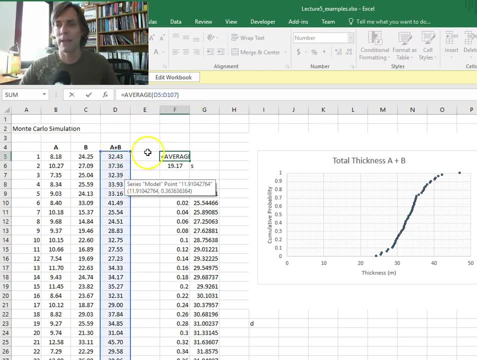 using Monte Carlo simulation from both formations A and B that are independent from each other. Now, if I want to calculate any type of summary statistics, Excel gives me an average. I can go ahead and highlight that set of values. I've highlighted them all. 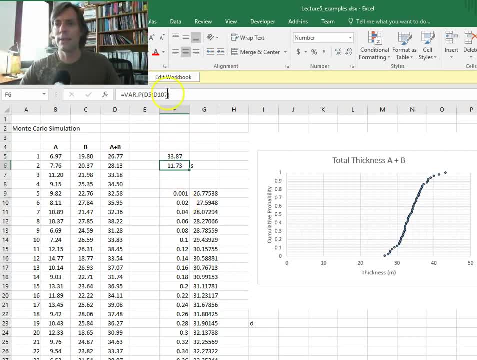 And I get an average of about 33.. I want the variance And I should calculate, probably, the variance of a sample, And if I go ahead and calculate that variance using the variance of the sample command, I will get something on the order of about 20.. 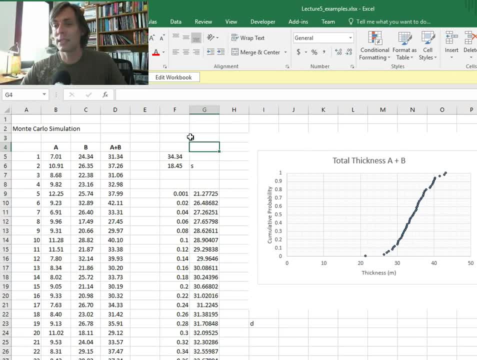 Now notice, every time I hit enter, those numbers are dancing around a little bit. They're not changing too much. Now what can we do to stop them from changing so much? You could use a lot of realizations Then the summary statistics would become much more stable. 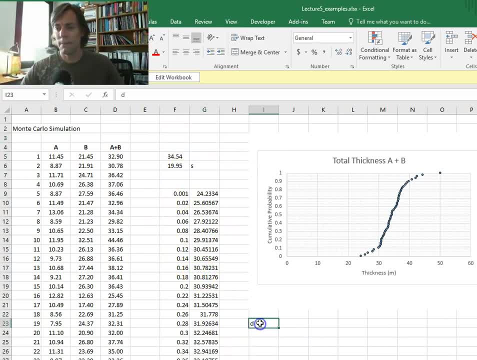 I also asked you for the P10 and the P90.. An easy way to do that would be to use the percentile command. I like using the EXC version. That assumes that the tails are unknown. What's the chance that you're going to sample the tails? 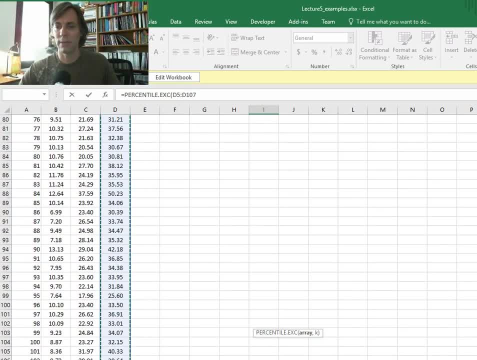 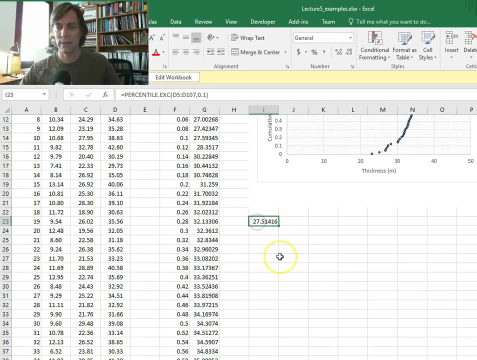 Now all we have to do is select the entire set of numbers And then we specify: we want the P10,, so 0.1. And we go ahead and we got 27 for that. We could copy that down. We just got to make a little move here. 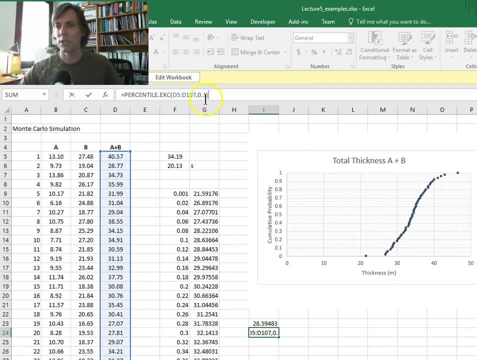 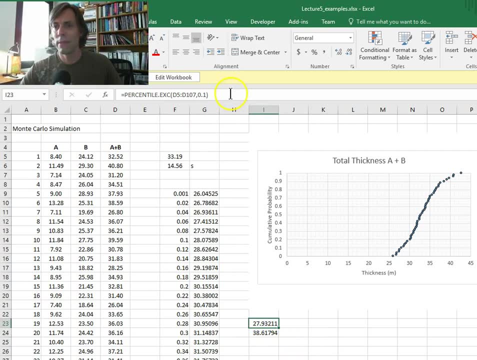 because it shifted down a little bit And we can change that to the 0.9.. And so now we have a P10 equal to 28,, 27 or so, and a P90 of about 40 for the number of meters thickness. 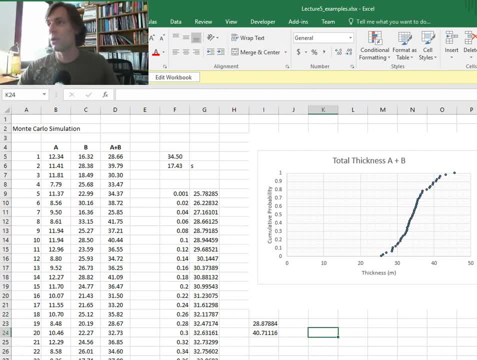 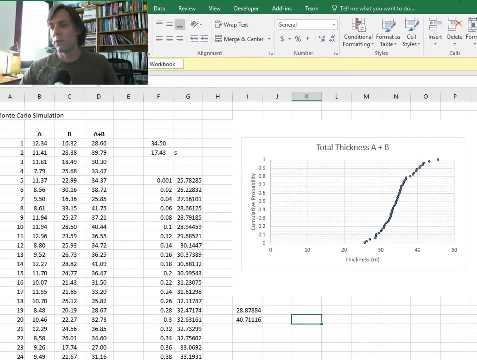 of the combined A and B units. So let's go ahead and we'll move that off to the side. Oh, You might wonder, I'll just explain one thing really quick. You might wonder. I have this distribution shown right here. What I did to calculate the CDF is I just simply calculated. 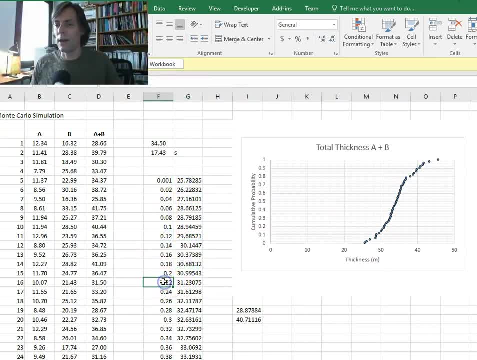 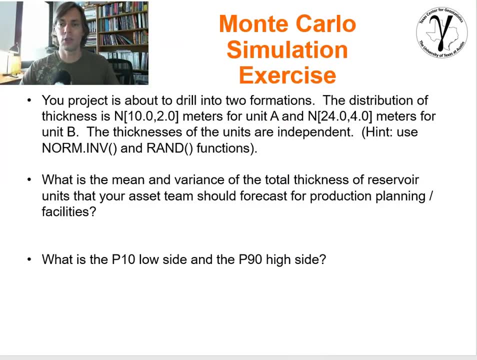 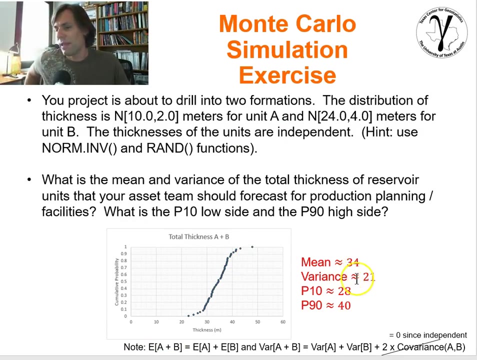 the percentiles for a whole bunch of different P values And then I just plotted them to get the full CDF of the output distribution. So I show that plot right here. The answer is a mean of about 34, a variance of about 21,. 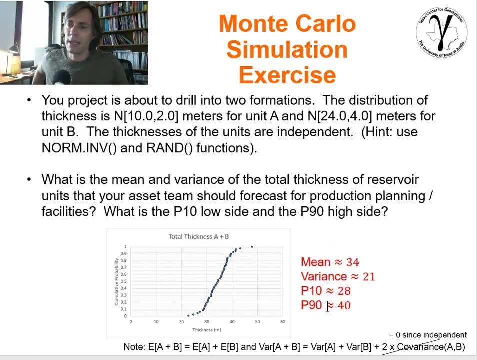 and the P10 and the P90.. And the P90 is shown right here. Now let me just- I'll just say it with words- The mean. let's recall when we talked about expectation: The expected value of A plus B was equal to the expectation. 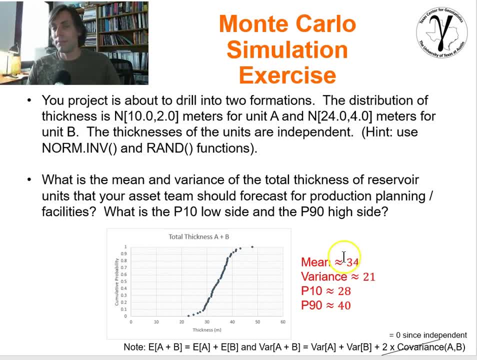 of A plus the expectation of B. The expectation operator has a distributive property to it, So we can do that. Okay, The mean, or expectation of a Gaussian distribution with a mean of 10 is 10.. The mean expectation: the expectation of a distribution. 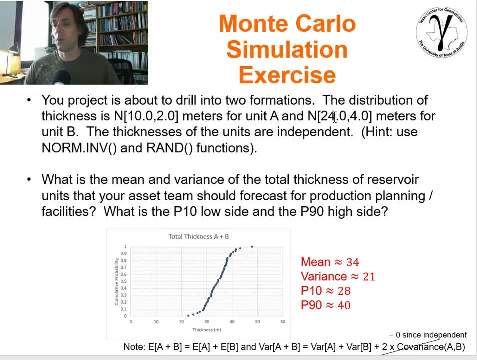 of a Gaussian distribution of a mean of 24 is 24.. And if we add the two together, the expectation of A plus B is equal to the expectation of A 10, plus the expectation of B 24.. And that makes sense. 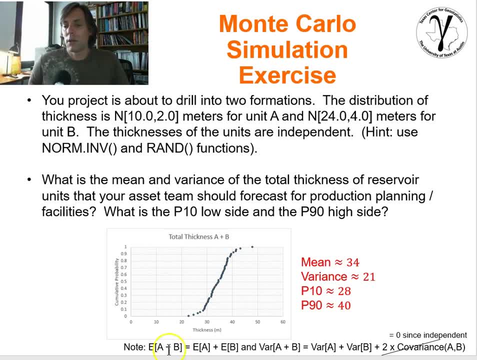 In addition to that, we could also look at the fact that variances tend to be- and I showed that right there- variances are additive. also, The variance of A, a random variable A plus a random variable B is equal to the variance of A plus the variance of B. 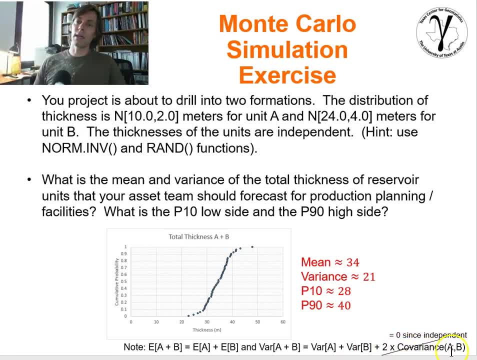 plus two times the covariance between A and B. By design, we set the correlation or covariance between A and B to be 0. We did not put one in, And so in fact we're in a situation now where we can just add those two variances together. 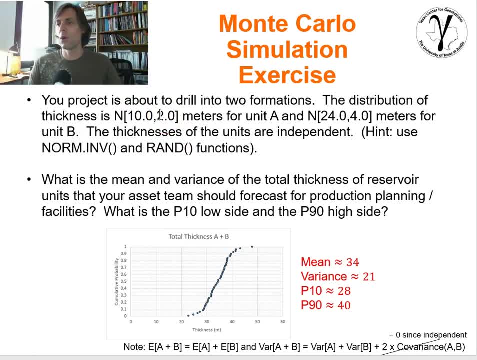 The variance of this first distribution is the square of the standard deviation 4.. The variance of this one square of the standard deviation of 4 is 16.. 4 plus 16. Is about 20 or so. You know there's going to be some oscillation in the statistics. 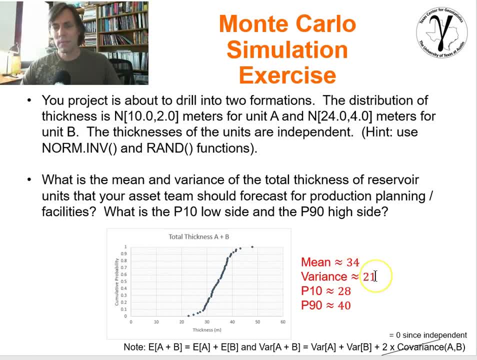 when we do sampling. So I say, or so We got 21.. So in general it holds. We also had a few samples. Maybe there was some artificial correlation between the two for the small sample size, So in this case we could have predicted the resulting distribution from the two.